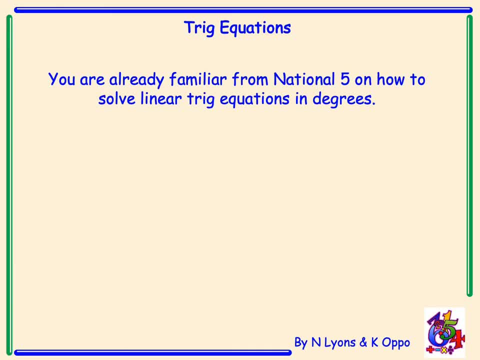 You are already familiar from National 5 on how to solve linear trig equations in degrees. 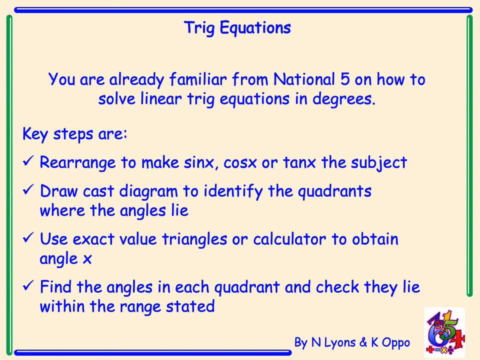 There are some key steps that we have to follow. We need to make sure we rearrange sine, cos or tan x to make them the subject. We need to ensure we have a cast diagram drawn to identify the quadrants and where the angles lie. We have to either use exact value triangles or a calculator to obtain the angle x and then finally find the angles in each quadrant but it's important that we check 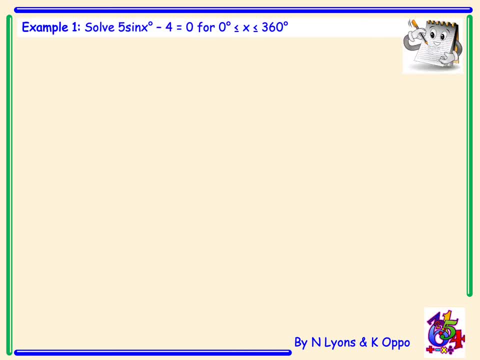 they lie within the range that is stated. Example 1. Solve 5 sine x minus 4 equals 0 for the x line between 0 and 360 degrees. 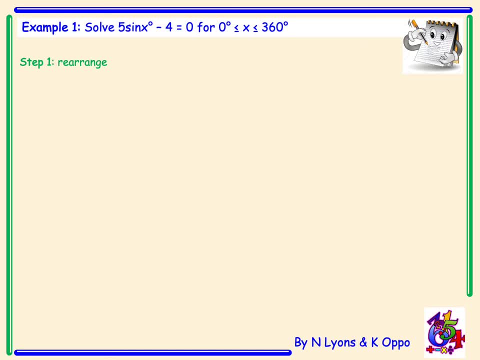 So the first step is to rearrange. So 5 sine x minus 4 equals 0 will become 5 sine x equals 4 and then if we divide by 5 we have sine x equal to 4 fifths. 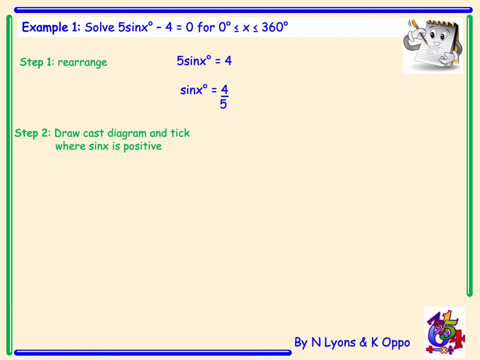 From there we will draw the cast diagram and we'll ensure we tick where sine x is positive because we have sine x equal to positive 4 over 5. So sine is positive in the first and the second quadrant. 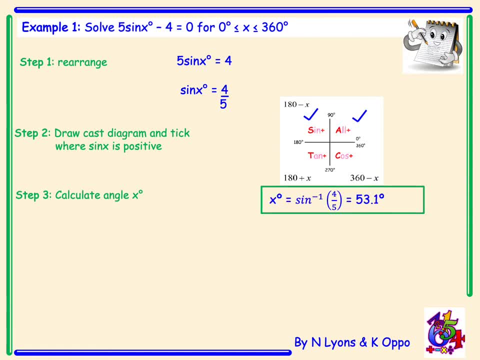 Next, we're going to calculate the angle x. To do that we need to do inverse sine of 4 fifths using a calculator and that gives us an answer of 53.1. The 53.1 degrees is the angle in the first quadrant 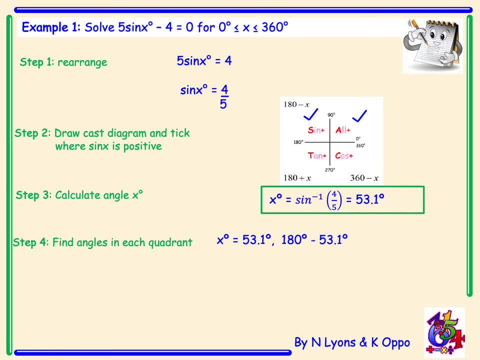 however the angle in the second quadrant we need to obtain by doing 180 take away 53.1. So our final solution for x is 53.1 degrees and 126.9. 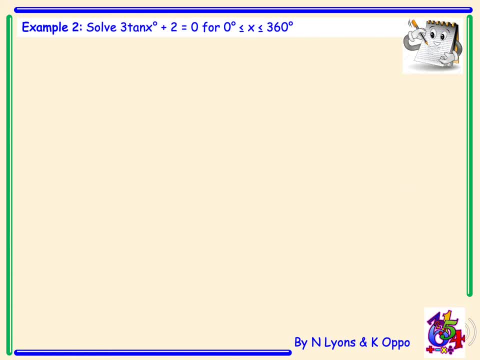 Example 2. Solve 3 tan x plus 2 equals zero for x between 0 and 360 degrees. Course Ti now is done. Then we name the subject. 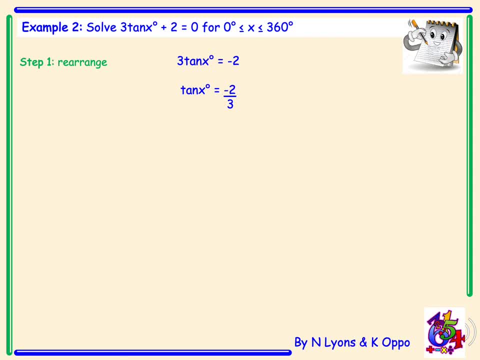 Our first step were going to do theordan words but we're also going to take an operation. 3 tan x plus 2 equals 0 pots over and divide x between 0 and 360 degrees. So that x equals negative 2. So we make our tan x a subject, so we'll take a plus 2 over and subtract it to get 3 tan x power is equal to negative 2. And then the three we'll come over and divide. Change aside, change the operation. 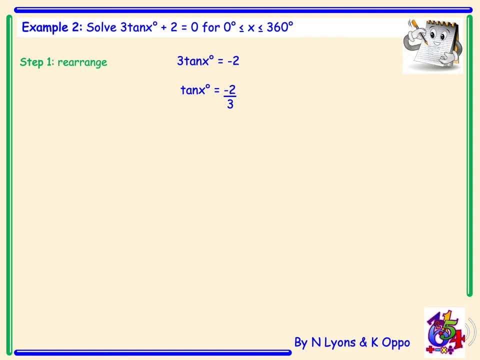 So for this we have to reject x over x times 3. Or suspension plug number 3. And then the second care should be the equation. We need a return per constant out of the future tier this again, equal to negative 2 over 3. Step 2, we then have to draw a cast diagram and we are going to tick where tan is negative. So our tan graph is negative in our second quadrant between 90 and 180 and it is also negative in our fourth quadrant at between 270 and 360. Now in order to work out the angle in each of these quadrants we need to know what the angle x is. So we'll do inverse tan of 2 over 3 which gives us 33.7. So that's step 3, calculating the angle x which is 33.7 and what we will do is use that to give the angle in each quadrant. So in the second quadrant there it'll be 180 minus 33.7 degrees. So So 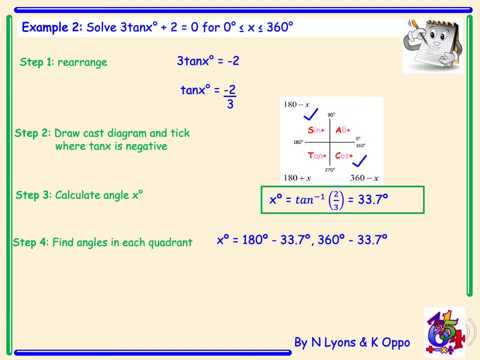 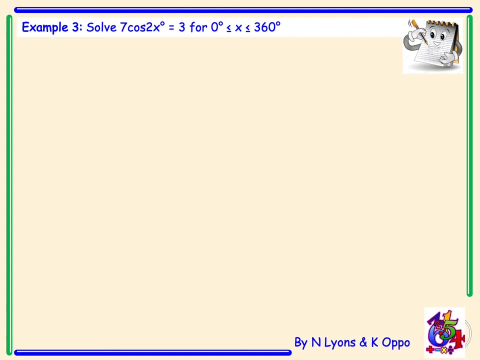 our fourth quadrant it will be 360 minus 33.7 degrees and this gives a final solution of 146.3 degrees and 326.3 degrees. Example 3. Solve 7 cos 2x equal to 3 for x line between 0 and 360 degrees. 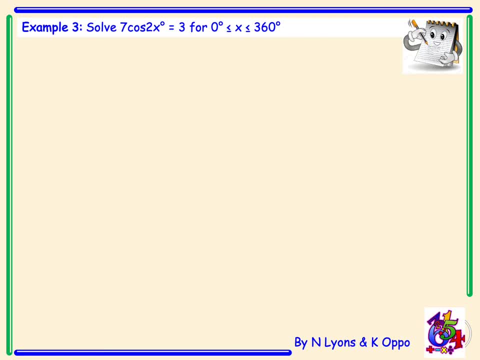 So the first step is again to make cos 2x a subject so we'll take our 7 over and divide and we'll get cos 2x is equal to 3 over 7. Now this is slightly different from our previous examples. Our previous examples had 1x which meant there was one wave and when we have one wave that means we have two angles but here we can see we have a 2x. Now that means we have two waves between 0 and 360. Therefore the equation is going to be 0 and 360. So we're going to have a 2x and we're going to have a 2x. 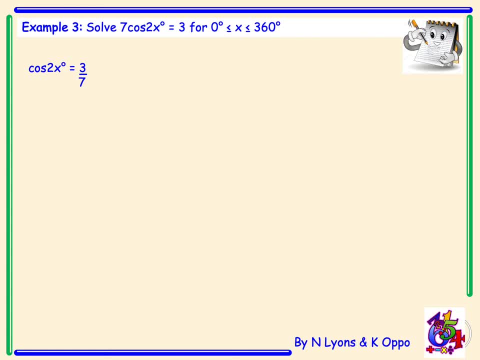 So we're going to have a 2x and we're going to have a 2x. So we're going to have a 2x and we're going to have a 2x. There will be four angles that we need to calculate. So there's four places that cos 2x is equal to 3 over 7. Next is we'll draw a cast diagram and we are going to tick the first and the fourth quadrant because cos is positive in these quadrants. Next step is we do have to do inverse cos of 3 over 7 and if we do that using a calculator we'll get an answer of 64.6 degrees. Now that is the angle in our first quadrant or that is what 2x is equal to. So we've got 2x is equal to 64.6 degrees and the angle in the fourth quadrant we'll do 360 minus 64.6 degrees to get 295.4 degrees. Now these two angles here are for the second quadrant. So we're going to have the first wave but remember we have two waves. So in order to get the next two angles we have to add 360 degrees to each of these. So adding 360 to 64.6 will give us 424.6 degrees and adding 360 to 295 will give us 655.4 degrees. Now here we have four angles so we'll put 2x equal to 64.6, 295.4, 424.6 and 655.4. But we've not to solve for 2x it has to be 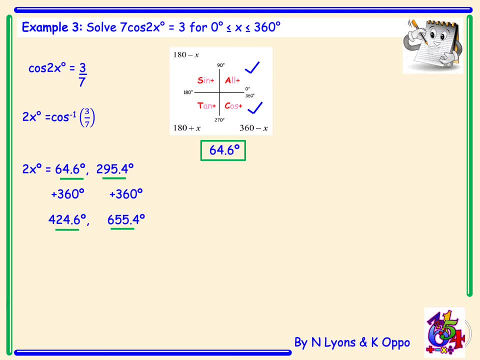 1x so we'll now divide each of these angles by 2 and doing that we get a solution of 32.3 degrees, 147.7 degrees, 212.4 degrees. Now we're going to have to divide each of these angles by 2 so this is the angle that we've got here. And this is the angle that we've got here. So we've got 2x 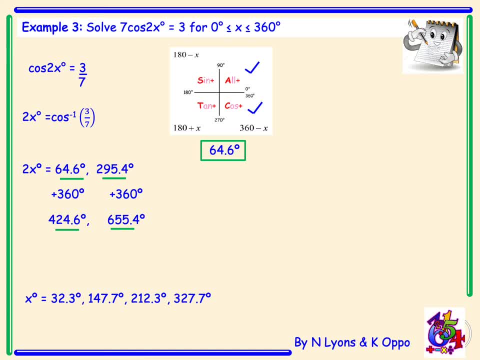 degrees and 327.7 degrees. That's four places, four angles where cos 2x is equal to 3 over 7 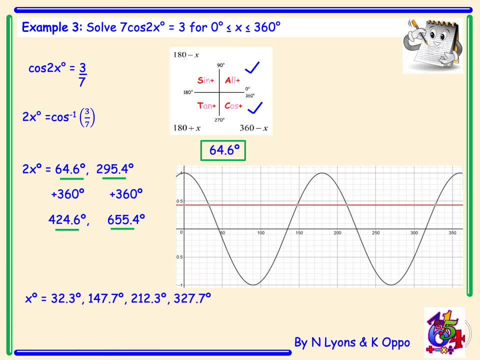 and here is the graph just to show you and the four angles are indicated as well. 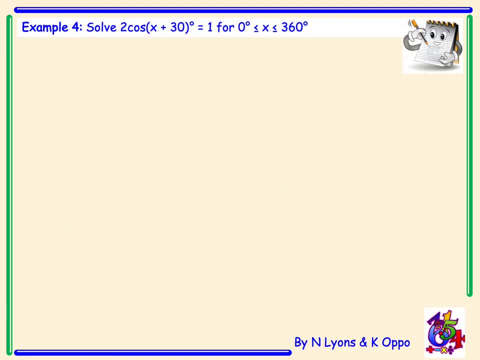 Example 4. Solve 2 cos of x plus 30 equal to 1, again for x lying between 0 and 360. 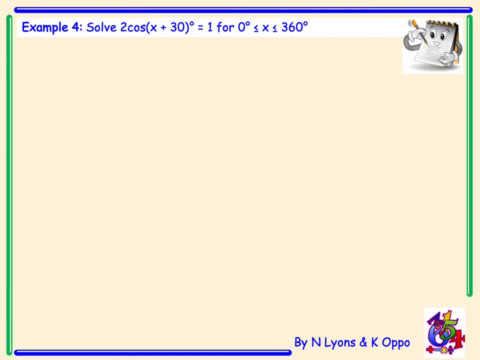 So from our functions and graphs unit at higher, we know that if we have 2 cos of x plus 30 degrees, the plus 30 essentially means that the graph has been shifted 30 degrees to the left. We also can note that if it's two cos, that means the graph will go up and have a maximum of two and a minimum of minus two. So the first thing we're going to do is rearrange and we'll have cos of x plus 30 equal to one half. From there we need to draw our cast diagram and we've got this equal to 1. 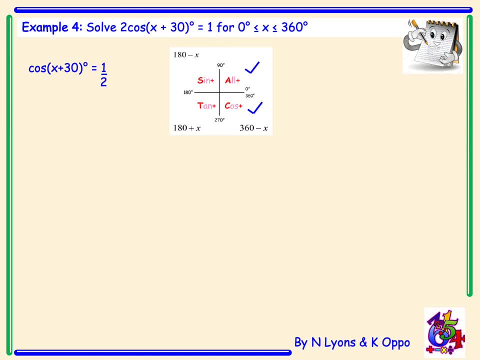 a positive a half so we tick where cos is positive so cos is positive in the first and the fourth quadrant from there we need to find inverse cos of one half which is 60 degrees therefore the angle in the first quadrant is going to be 60 degrees and the angle in the fourth quadrant will be 360 minus 60 which is 300. now that's x plus 30 degrees gives us these two angles therefore we need to take the plus 30 over and subtract and then we have a final answer of x equal to 30 degrees or x equal to 270 degrees again to show you a picture of what this would look like 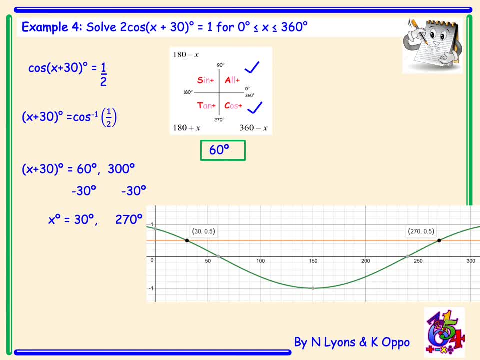 here the green curve is our cos graph and our yellow line there is um y equals a half we can clearly see that these two meet at 30 degrees one half and 270 degrees one half 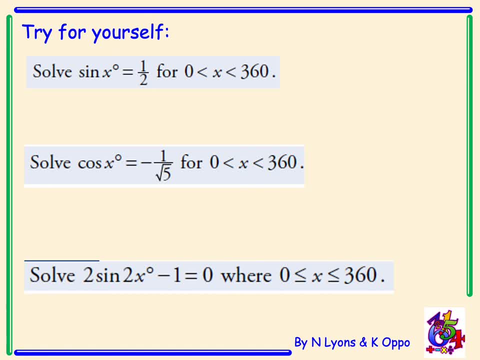 now try these examples for yourself please pause the video 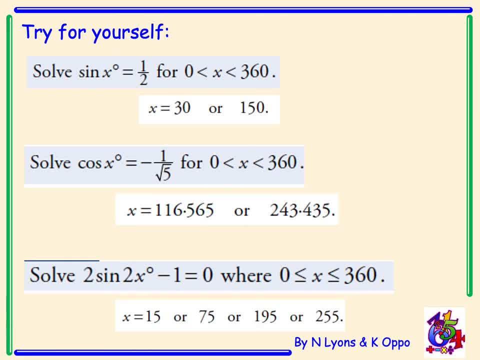 and the solutions are for the first trig equation x is 30 or 150 degrees for the second trig equation x is 116.565 or 243.435